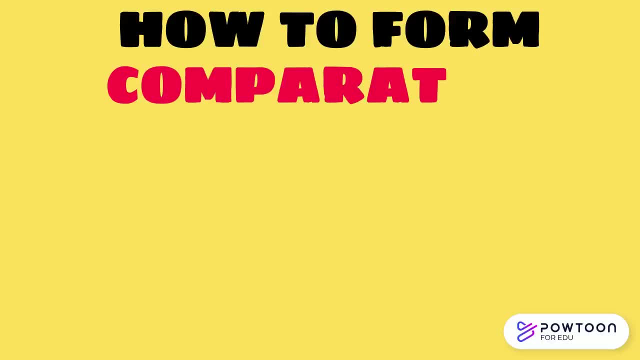 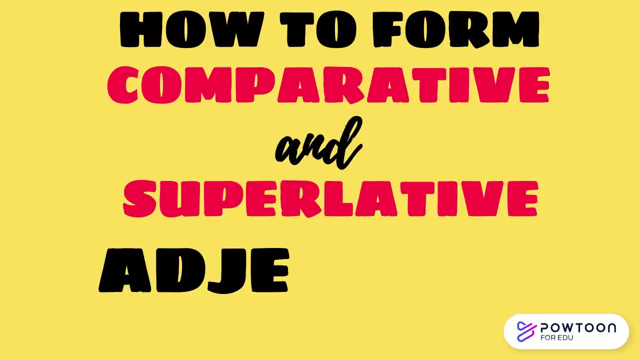 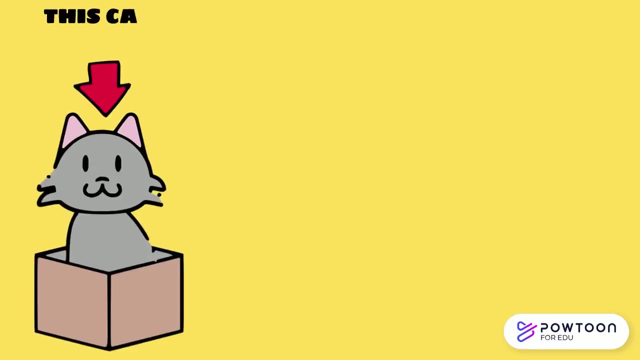 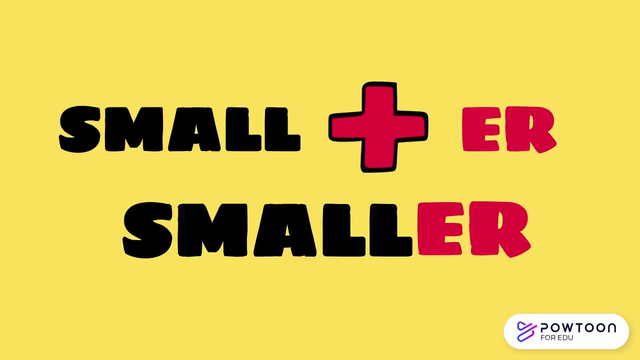 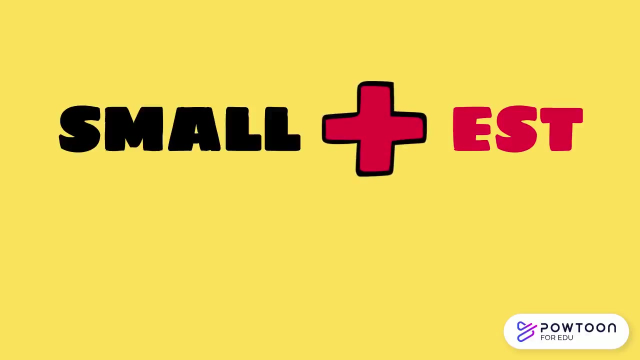 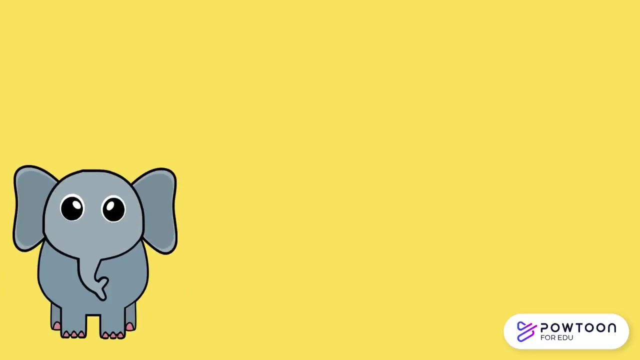 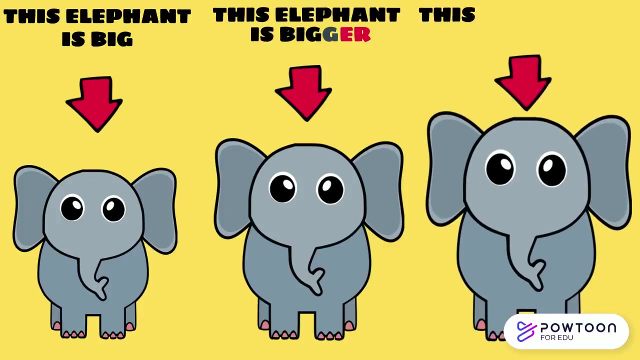 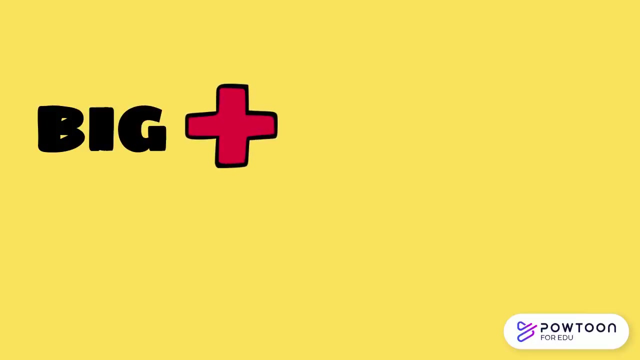 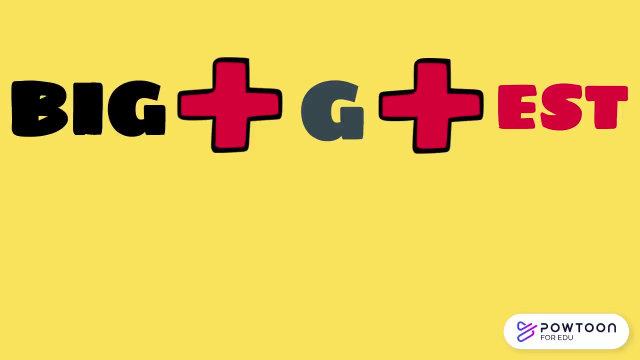 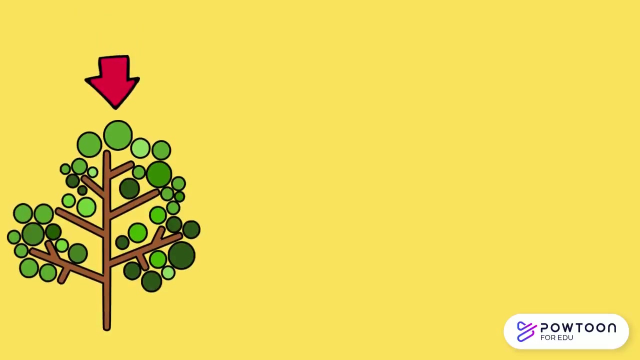 This cat is small. This cat is smaller. This cat is the smallest. This cat is the biggest. This elephant is big. This elephant is bigger. This elephant is the biggest. This elephant is the smallest. This tree is beautiful. This tree is beautiful. 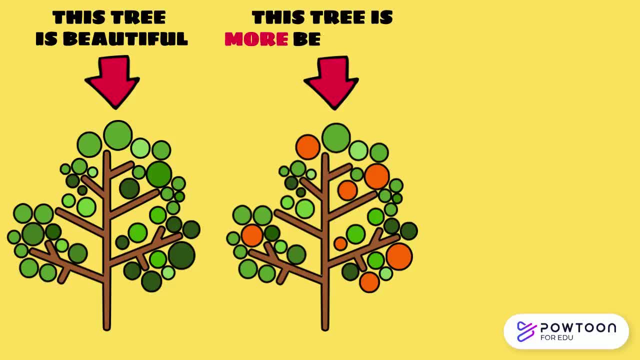 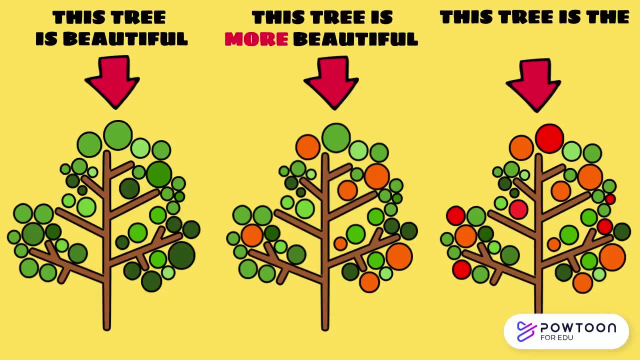 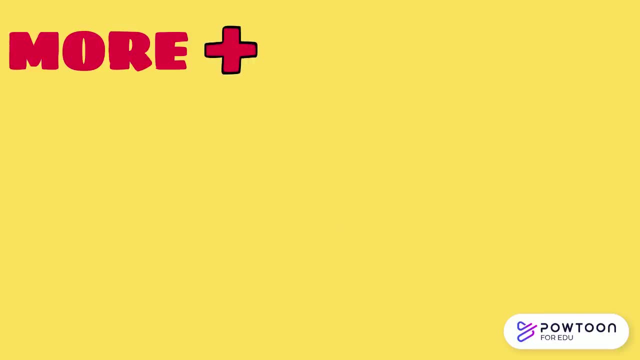 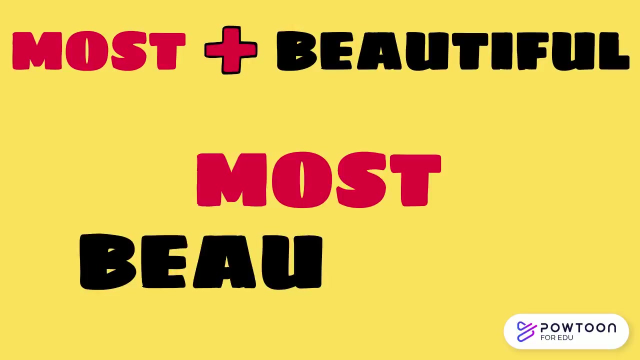 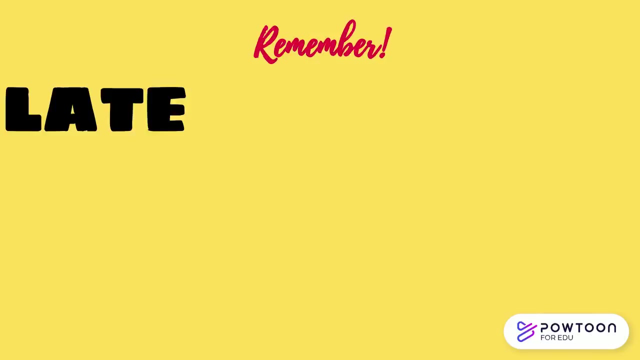 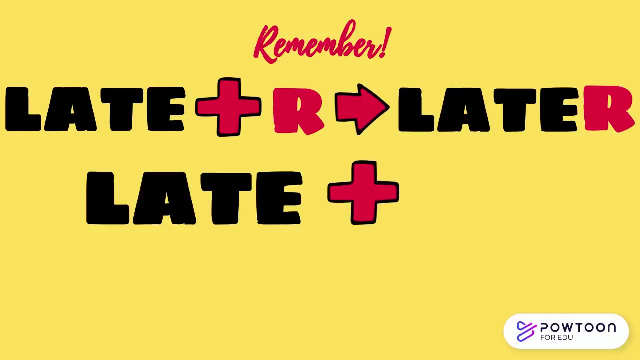 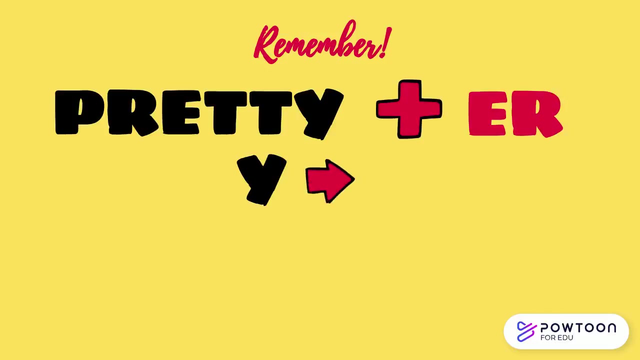